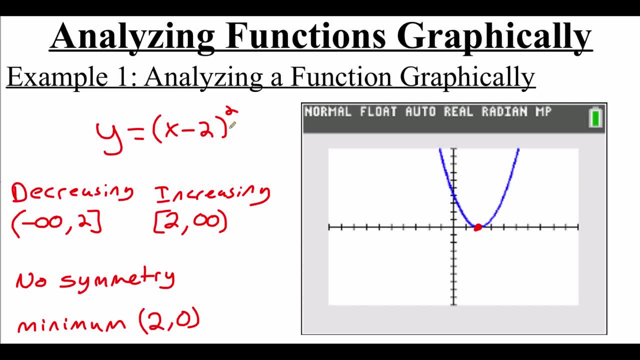 And one other thing that we should recognize is that this graph is a parabola, so it's very similar to the graph of the equation y equals x squared. Normally, our parabola for y equals x squared is centered at the origin, but this one got shifted to the right two spaces. 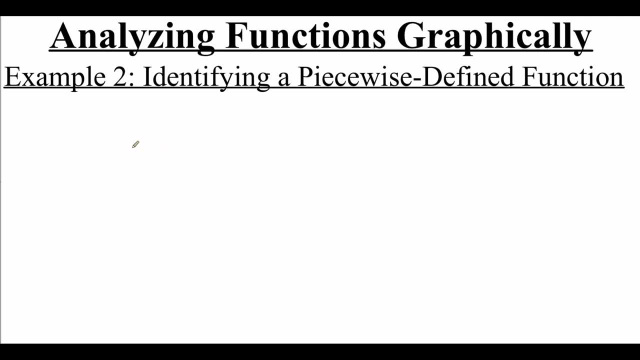 In this example we're going to look at talking about piecewise defined functions. So I want to look at the function f of x equals the absolute value of x. But I want to look at this function just a little bit differently Now. a piecewise defined function is a function that's made up of multiple other 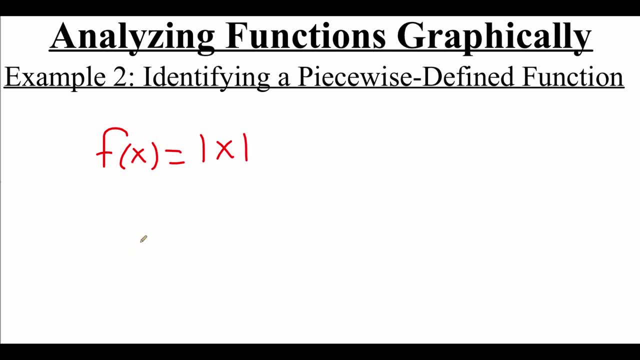 functions over specified domains. So we can really think about this absolute value function as kind of a combination of two separate functions. The first function- if we're looking at the absolute value of x, then the first piece would just be: f of x is equal to the absolute value of x. 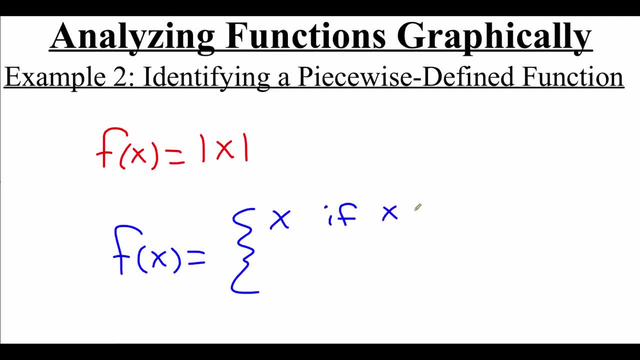 Now f of x is equal to the absolute x if the x values that we're plugging in are greater than or equal to zero. Because if we plug in any positive number, x, for our x value in this absolute value, the answer we get back is just going to be the exact same number that we plugged in Where we 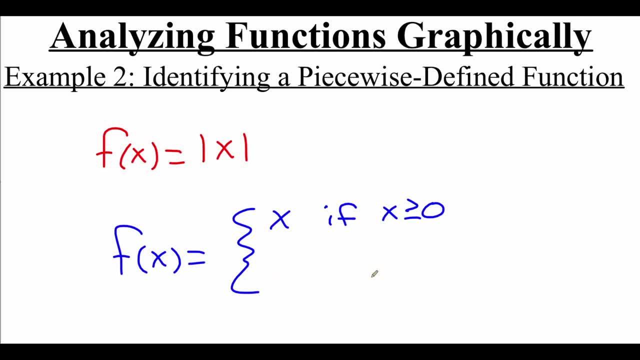 really have to be careful is with negative numbers. So if we have x values that are less than zero, then our function is going to be defined as the opposite of x. So like if we plug in, If we plugged in, negative seven here, the absolute value of negative seven is positive seven. 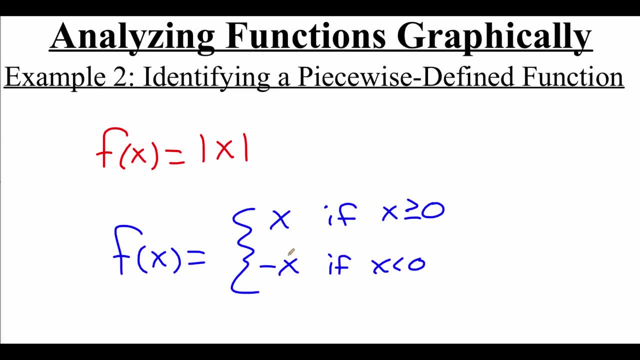 So we plugged in an x value that was smaller than zero and the answer we got back was the opposite of that original x value. So a piecewise defined function. like I said, it's just a function that's made up of multiple pieces over specified domains. 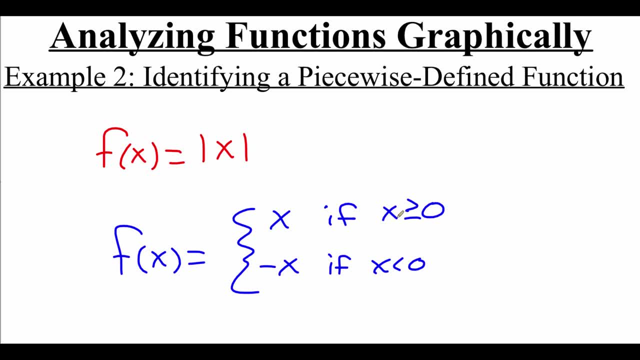 Now, when you start plugging values into a piecewise defined function, the domain will tell you what piece of your function to plug it into. So this top piece says: if we're using x values that are greater than or equal to zero, then we plug it into the top piece of the function. 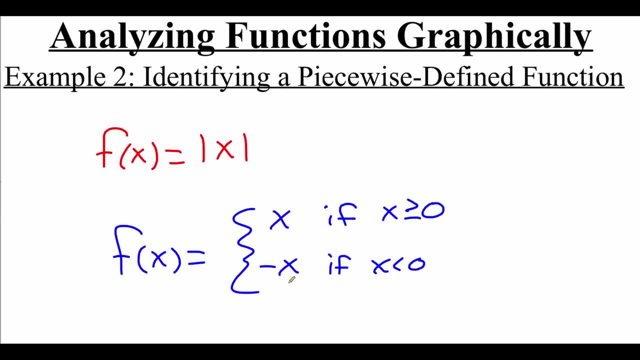 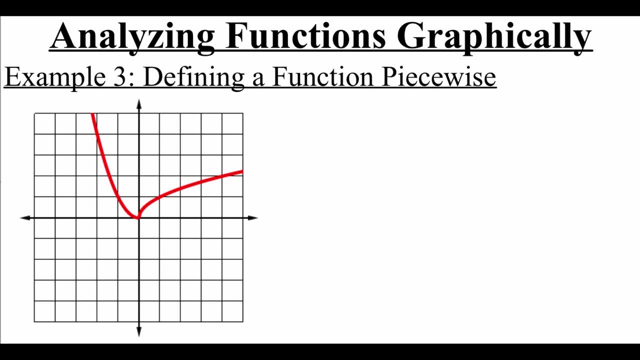 But if we're using x values that are less than zero, then we would plug those into the bottom piece of our function. Now, in this example, we're gonna take a look at that graph that's on the left-hand side of our screen there. 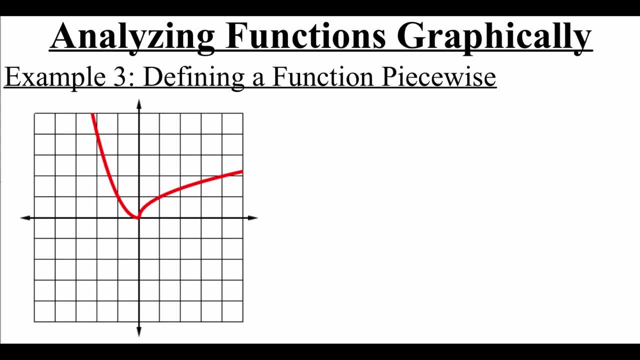 and we're going to try to write out a piecewise defined function for this graph. So I'm first looking at the left-hand side and that first chunk of my graph looks sort of like the left-hand side of a parabola, up until we hit that x value of zero. 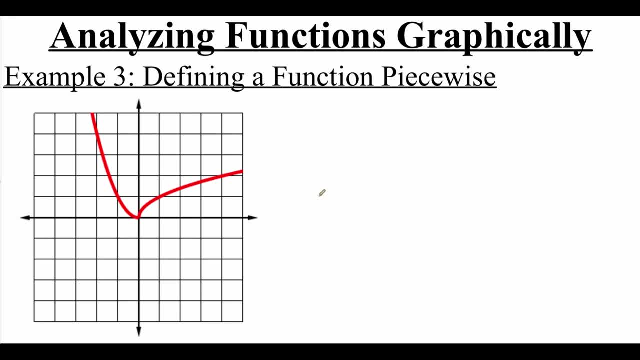 So that's actually how I'm going to start defining my piecewise function. So the left-hand side looks like x squared, and that's for x values that are less than zero. Now on the right-hand side, once we hit zero, this starts to look like a square root graph. 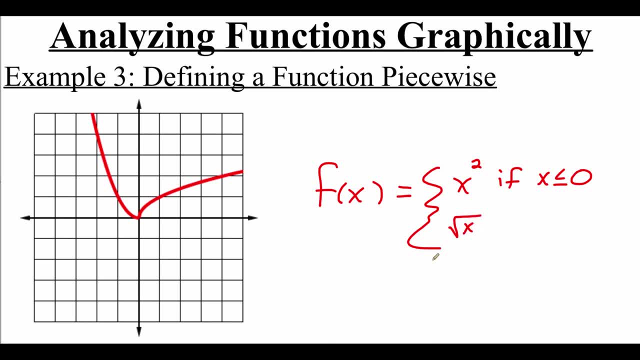 So that's how I'm going to define my second piece, And this is for x values on the right-hand side. So that's going to be for x values that are greater than zero. Now there is actually a way for us to type in: 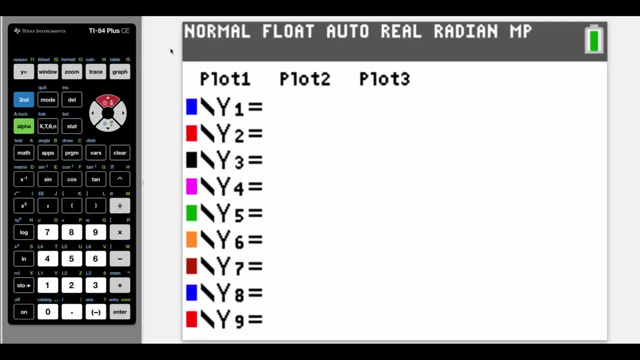 these piecewise defined functions on our calculator. So I'm in my y equals screen with my calculator and I want to type in that first piece that x squared for x values that are less than or equal to zero. Now what we're going to do is we're gonna take 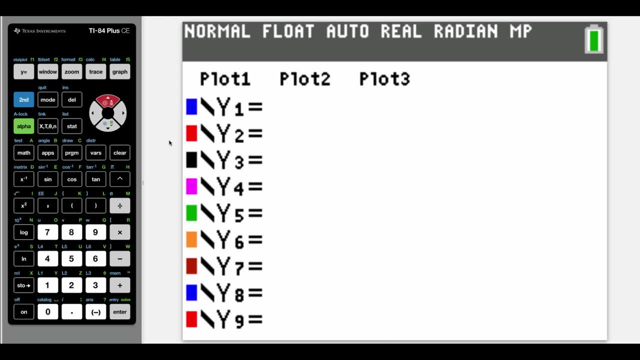 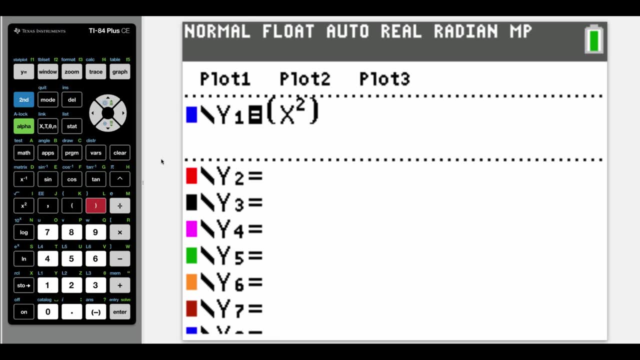 our function that we're typing and we're gonna put it inside a parentheses. So I'm gonna go parentheses and then x squared and then I'm gonna close up my parentheses. Now what we have to do to separate the function from the domain that we're going to enter in. 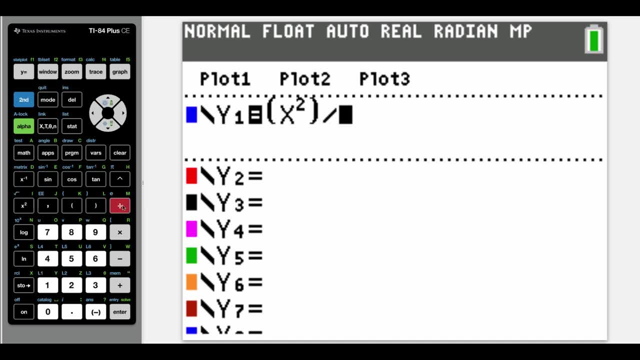 is hit our division symbol in there, and then we also need to put our domain inside of parentheses as well, So I'm gonna open another set of parentheses here. I want x values that are gonna be less than or equal to zero. So we need to find our inequality symbols. 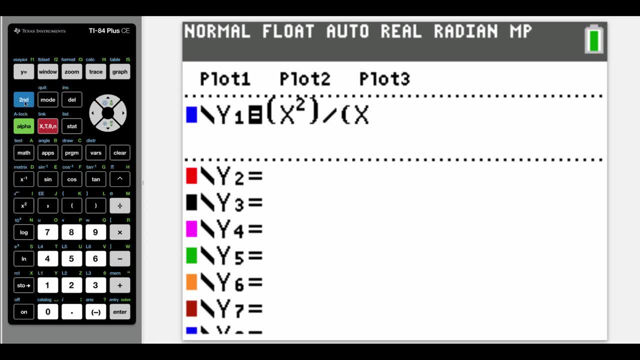 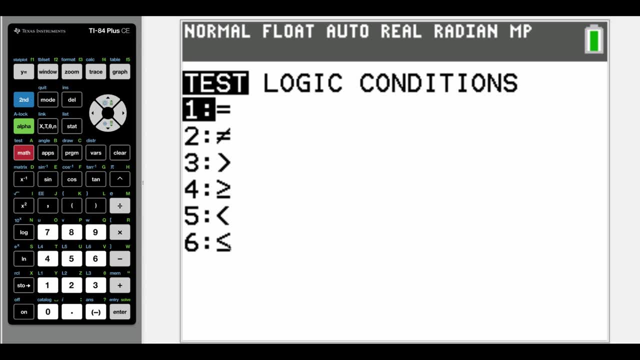 and right above your math button it says test. So I'm gonna go second math to open up that test menu. and we wanted x values that were less than or equal. So we want option number six, down on the bottom: x values that are less than or equal to zero. 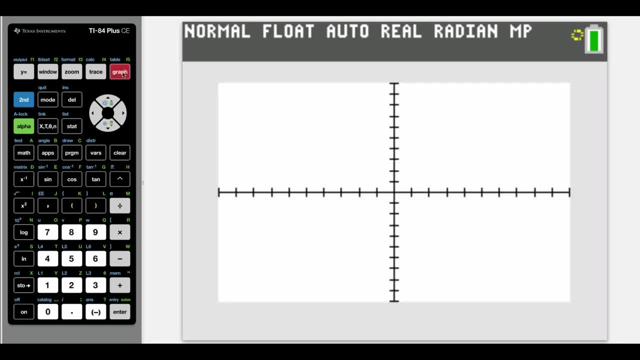 and then we close up our parentheses and then, if we hit our graph button, it'll only graph out that left hand side of our parabola until we hit that x value of zero. But we've got another piece of our function to add in here.